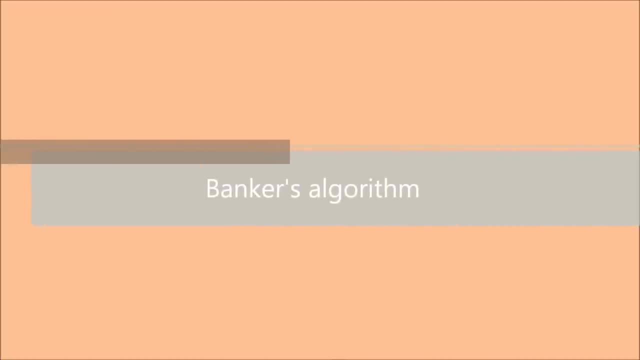 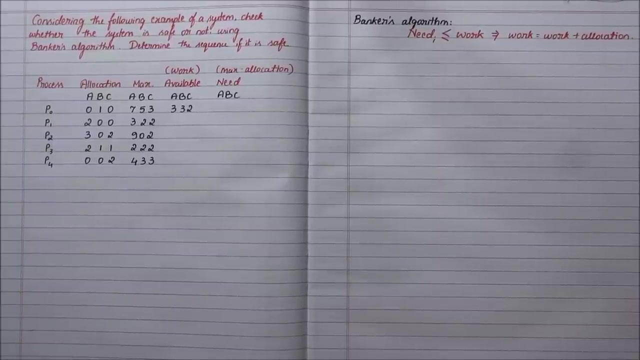 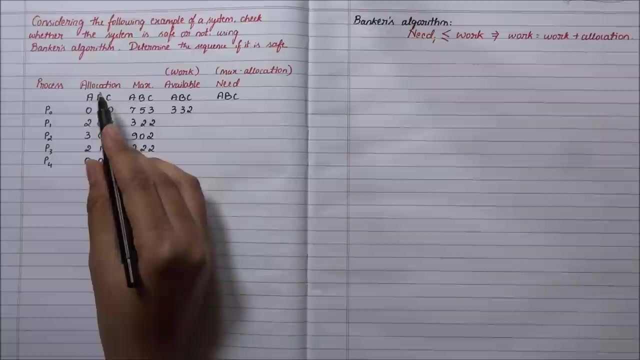 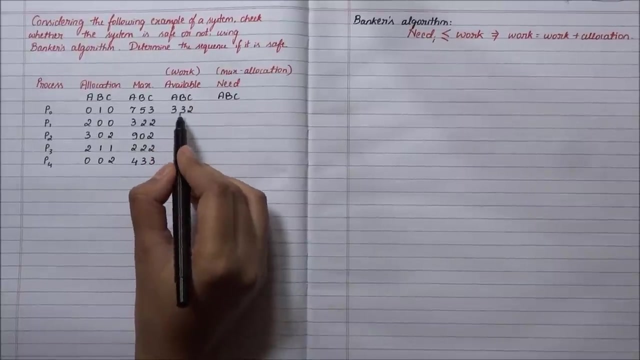 Bankers algorithm. It's one of the famous algorithms under the deadlock avoidance. Let's take an example of a system with five processes whose allocation and maximum is given and initially the work or available is 332.. We need to find out the need matrix by subtracting. 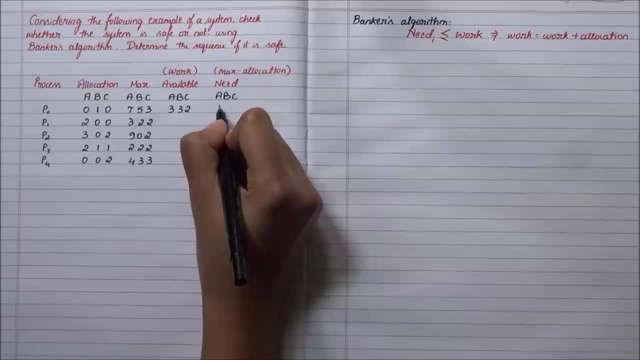 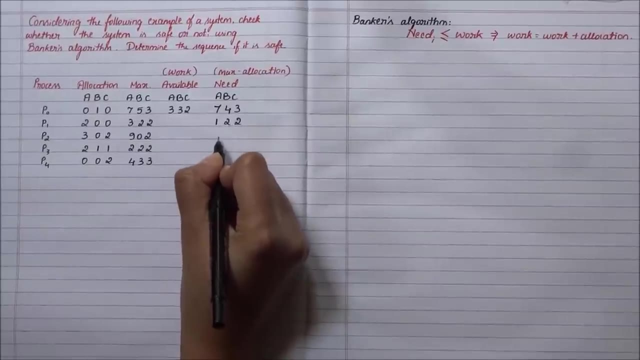 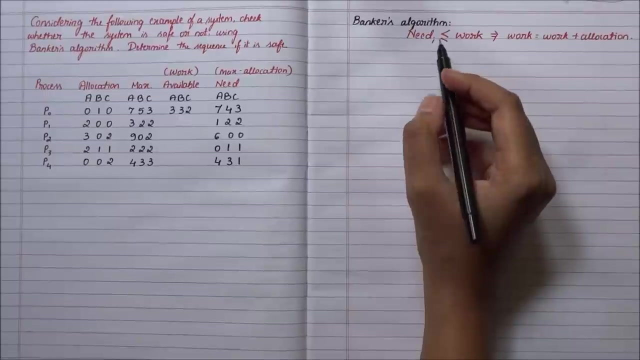 allocation from max, So it will be 7, 4, 3, 1, 2, 2, 6, 0, 0, 0, 1, 1, 4, 3, 1.. According to the algorithm, we need to compare the need of each process with the work. First, let me. 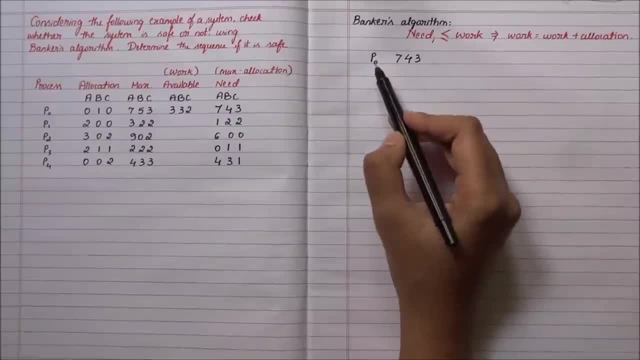 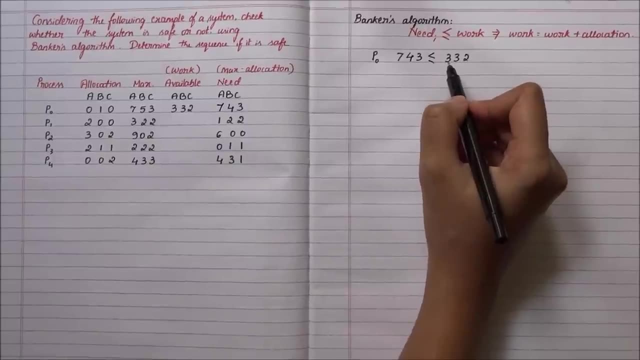 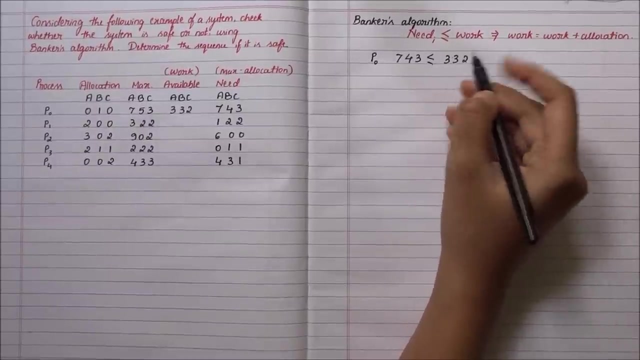 take up P naught. The need of P naught is 7, 4, 3.. So we should check if it's less than or equal to the work. Work is 3, 3, 2.. We should check if need is less than work. So it's clearly not less than or equal to work. So here the 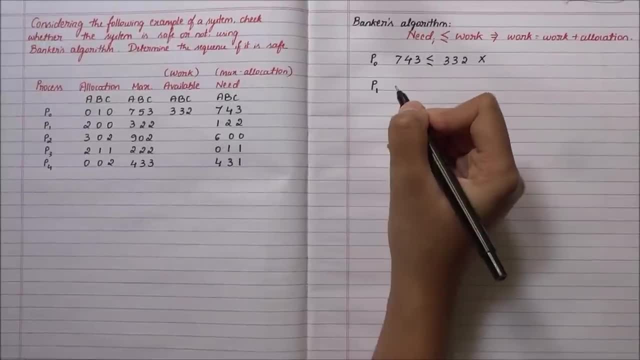 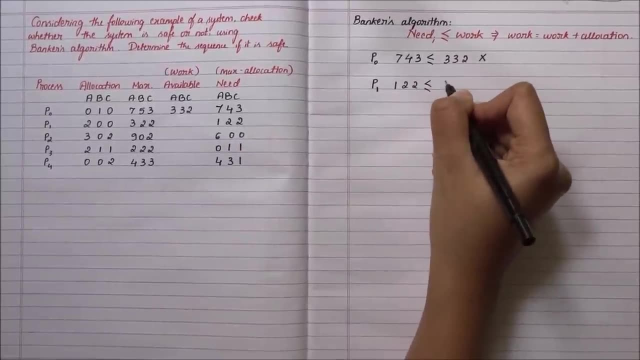 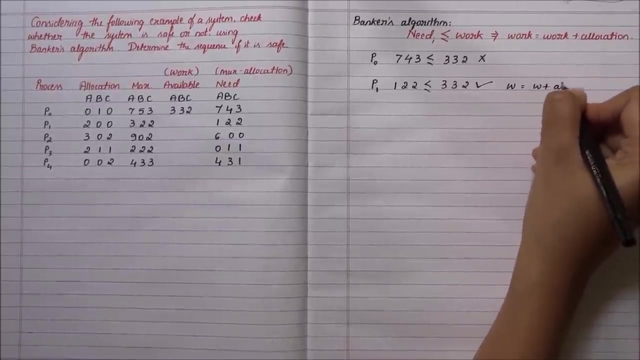 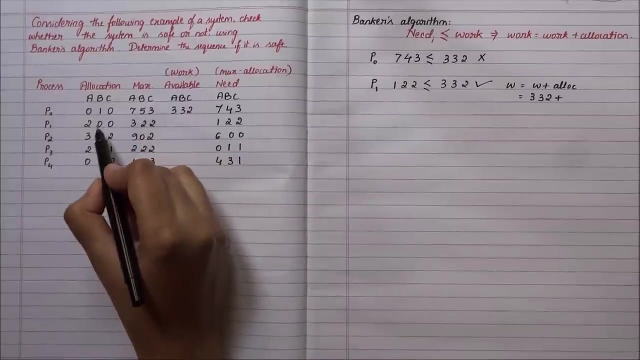 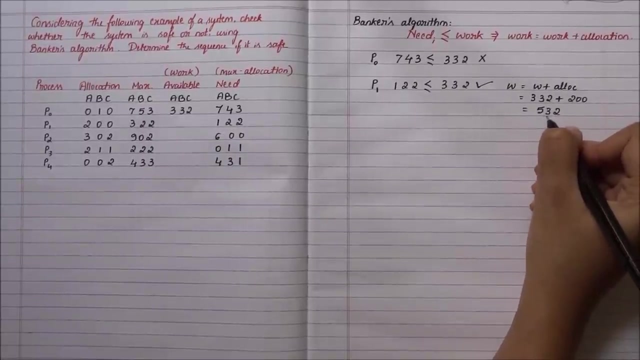 condition fails and we should check for the next process. Next process is P1, whose need is 1, 2, 2, which is less than or equal to 3, 3, 2.. This is true. The new work becomes work 3, 3, 2 plus. allocation of P1 is 2, 0, 0.. 5, 3, 2 is the new work. We need to update it in. 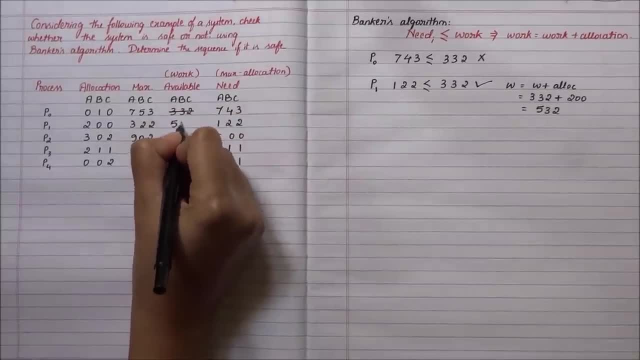 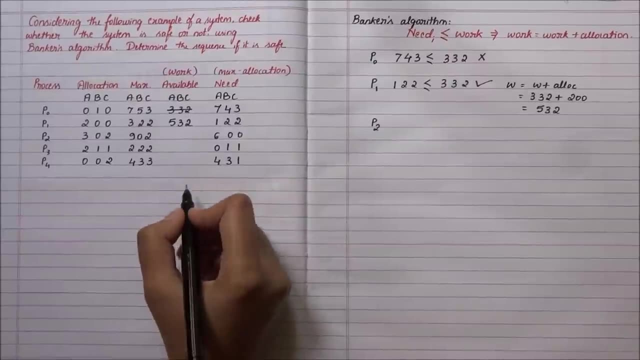 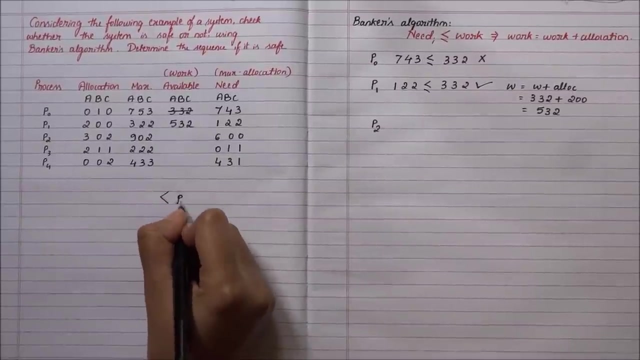 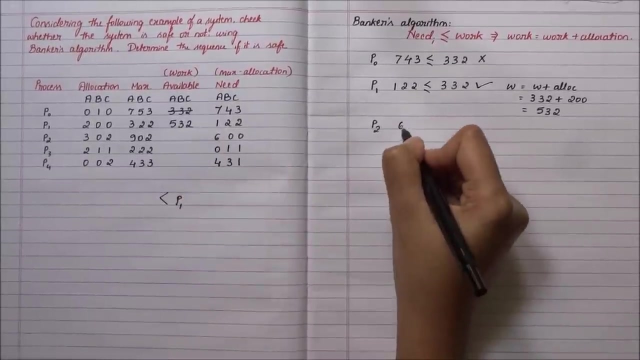 the matrix. Before going to the next process, we need to keep track of a safe sequence, of which are all the processes that have entered the safe sequence. Now P1 has just entered the safe sequence. Let me go for P2.. The need of P2 is 6 0 0.. 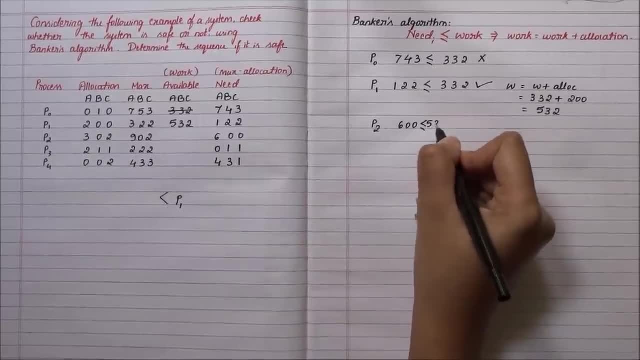 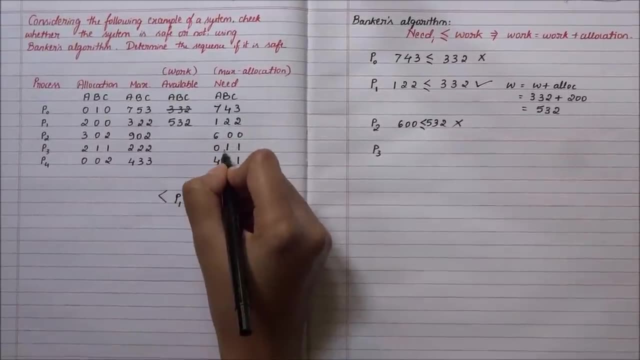 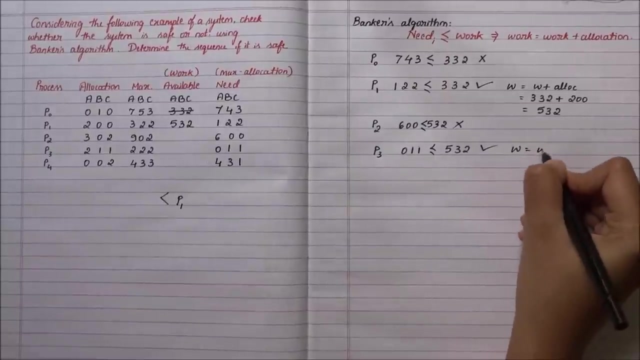 Less than or equal to, the new work is 5, 3, 2.. This is false. So let me go to the next process, P3, whose need is 0, 1, 1.. Less than or equal to 5, 3, 2.. This is true, So work becomes. 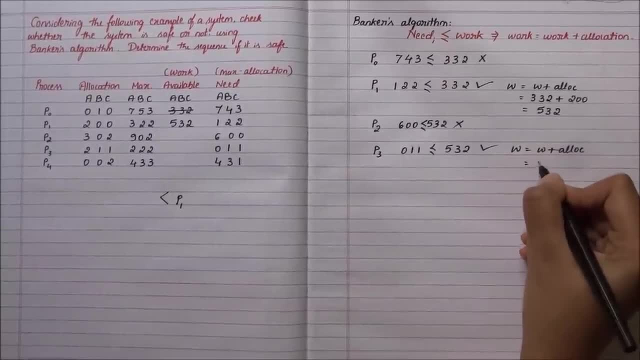 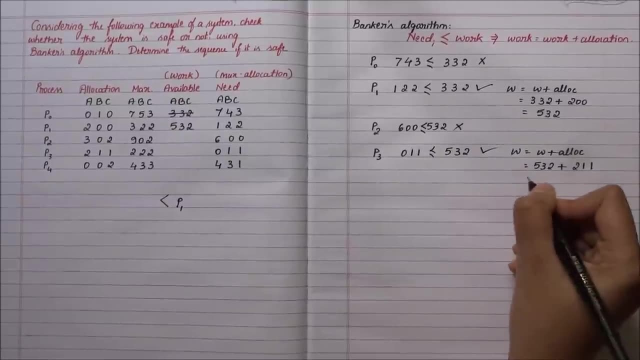 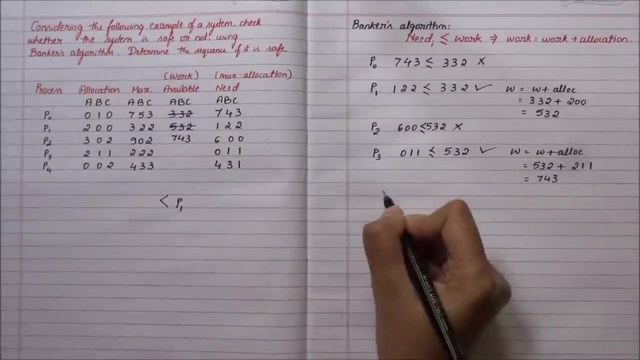 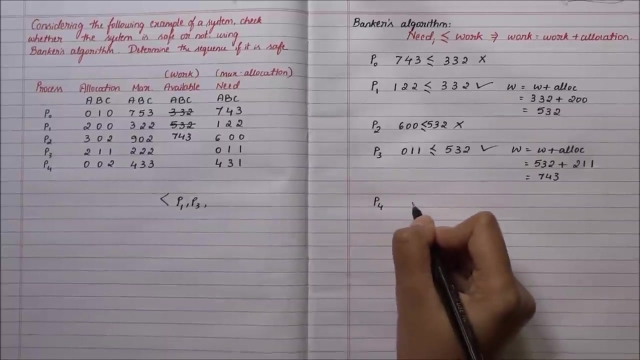 work plus allocation. Current work is 5: 32 plus allocation of P3 is 2: 1, 1.. So total it will be 7, 43.. This has to be updated here: 7, 4, 3.. And P3 has now entered the safe sequence. Let me go for P4. 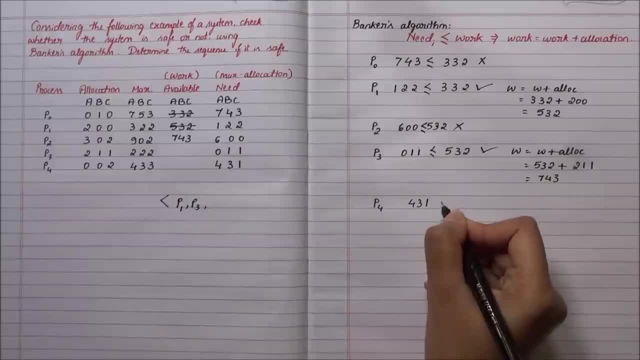 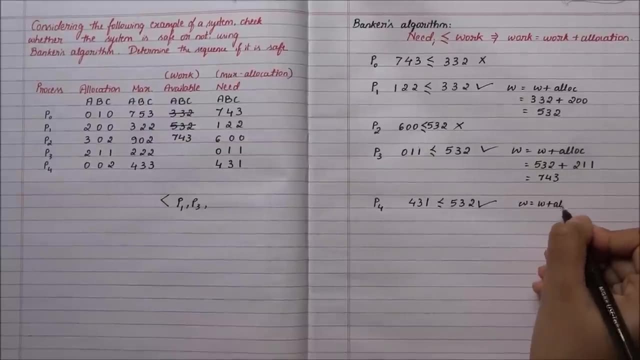 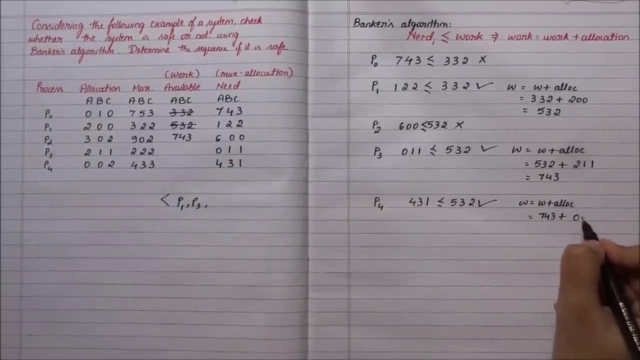 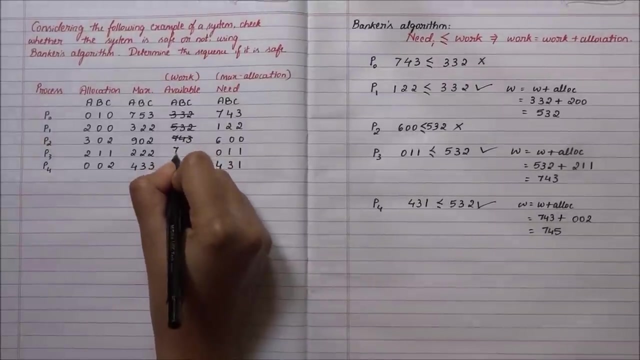 Need of P4 is 4 3, 1.. Less than or equal to 5 3, 2.. This is true, So work becomes work plus allocation. Work is 7: 43. Thus allocation of P4 is 0, 02.. It will be 7: 4, 5.. New work is 7: 4, 5.. And P4 has entered. 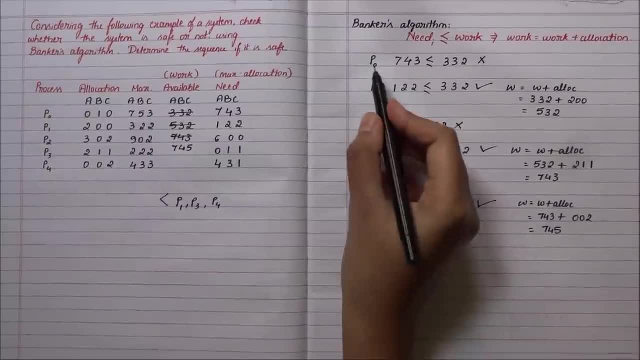 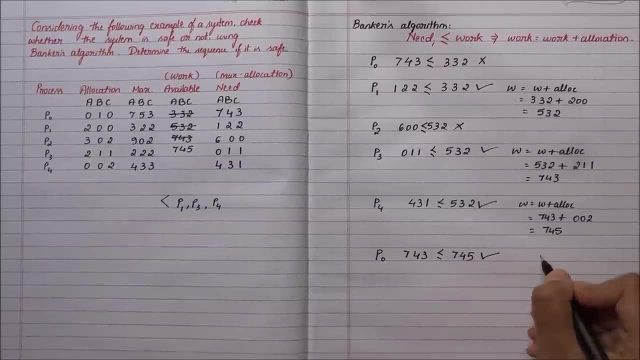 the safe sequence. Now, going back to P naught, P0 has need of 7, 43 less than or equal to 7, 4, 5.. this is now true. so work is equal to work plus allocation. work is 745 plus. 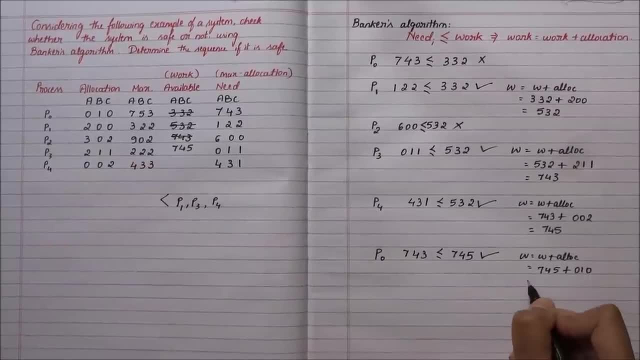 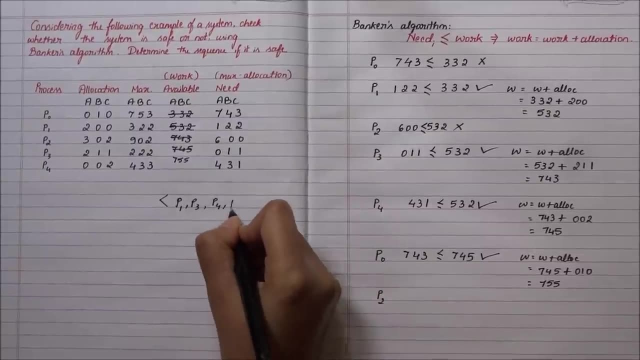 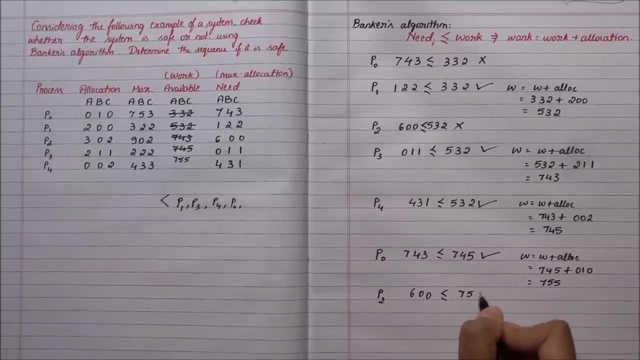 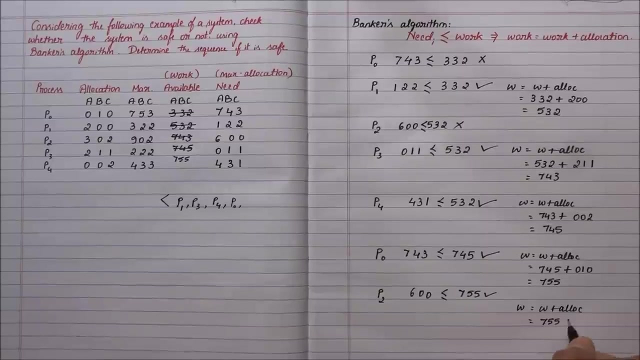 allocation of p0 is 010, total becomes 755. the new work is 755. p0 has now entered the safe sequence. need of p2 is 600 less than or equal to 755. this is true, so work is equal to work plus allocation. work is 755. allocation of p2. 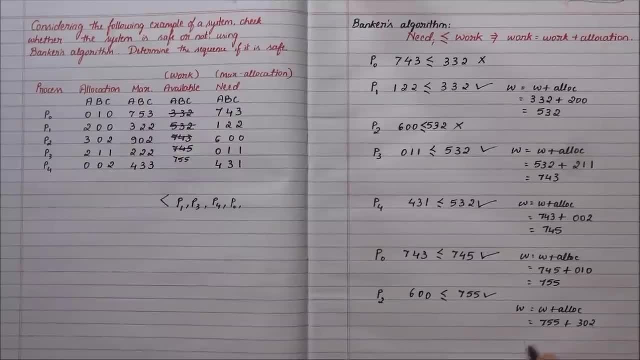 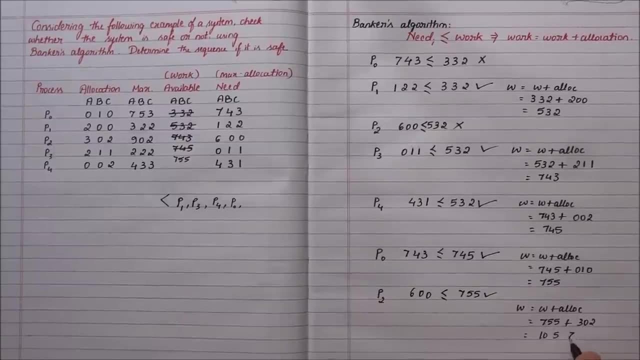 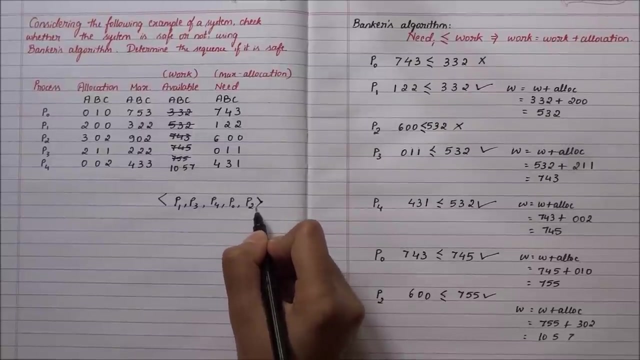 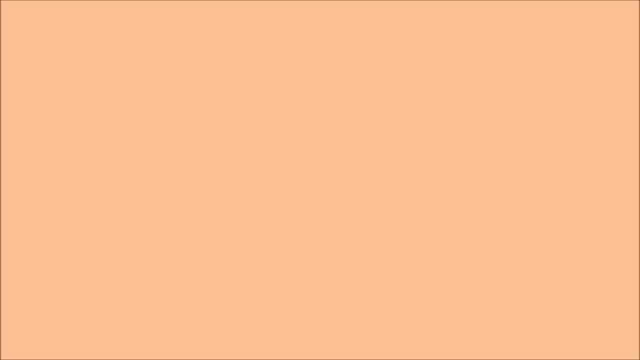 is 302, so in total it will be 7 plus 3, 10, 5 plus 0, 5, 5 plus 2, 7. this is the final work and at the end, p2 has also entered the safe sequence. this is the final work and at the end, p2 has also entered the safe sequence. this is the